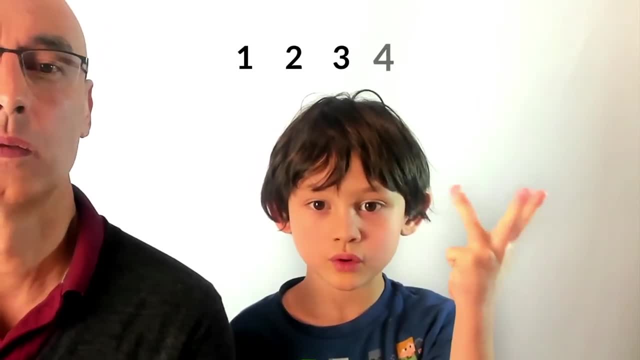 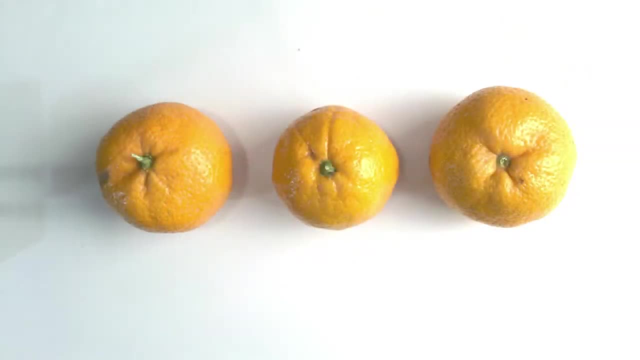 Yeah, One, two, three, four, five. Okay, awesome Five. So now I'm going to show you some objects. Do you like mandarins? Oh yeah, I want some. Well, you can actually eat these if you do a good job counting, okay. 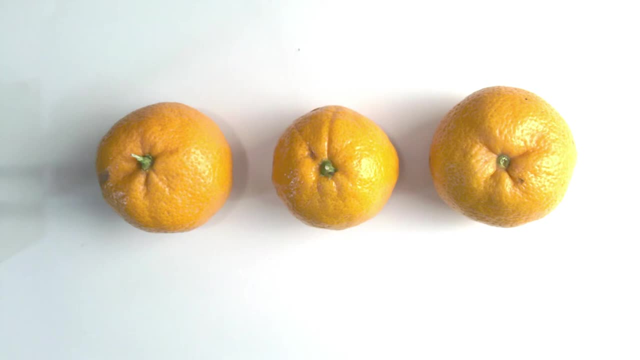 Okay, All right. So how many are there? Three, Okay. how do you know that? Well, I can see what it's, three, but I can make sure by counting. Okay, can you do that now, And while you're counting, then touch each mandarin. 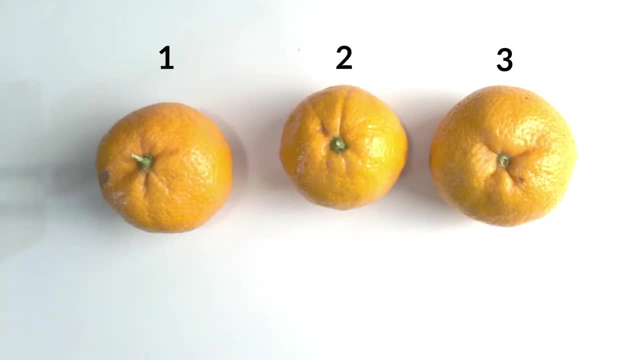 One, two, three. So what I notice is that the last number you counted was three, And that's how you know how many mandarins there are. Is that right? Yep, Okay, So the last number that you count tells you how many objects you have. 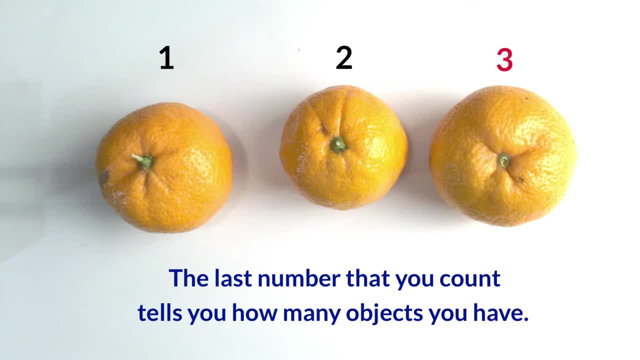 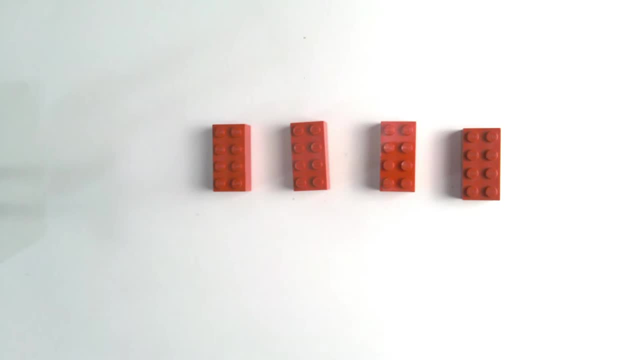 All right, So let's go ahead and try with something else. How about these? What are these Legos? Oh, I know you like that. I want to build with them. Okay, Why don't you count them first? Okay, so why don't you count them? 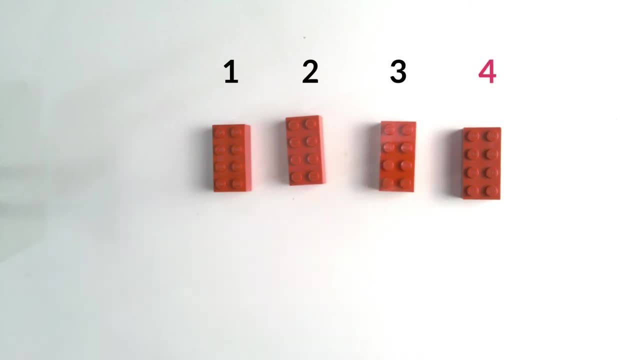 One, two, three, four, That was easy. Four Legos- Good job, Okay. And I bet you'd like to build something with those too right, Legos, Legos. So I've got a question. I've got a question for you. 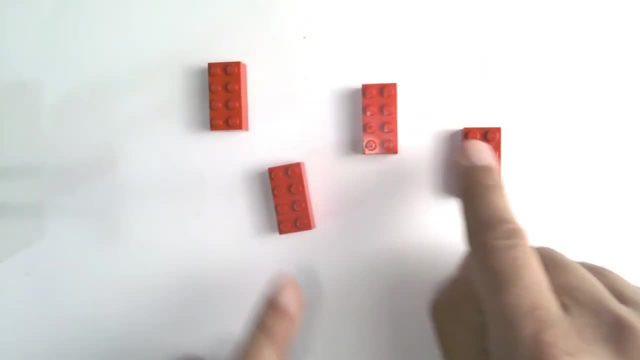 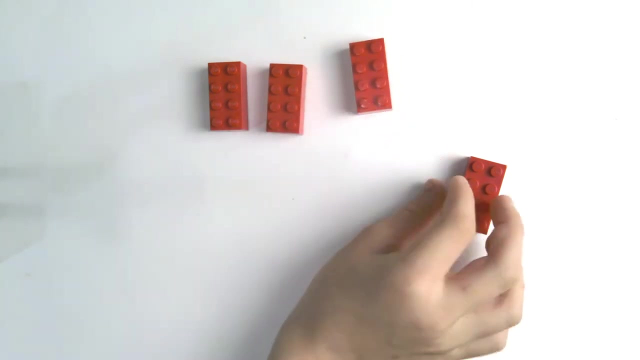 What is it? All right? So if I move them around a little bit, is that still four Legos? Yes, How can you be sure? Well, you can count. You can put them like how they were. There's a bunch of ways. 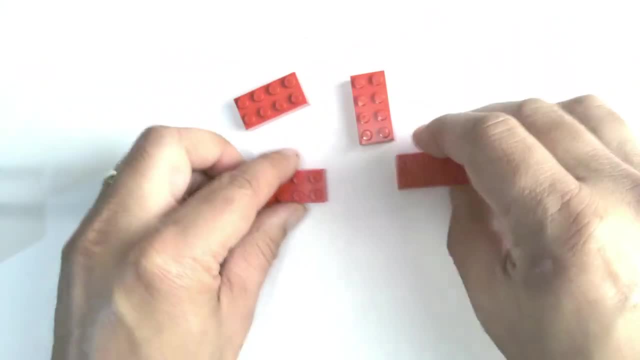 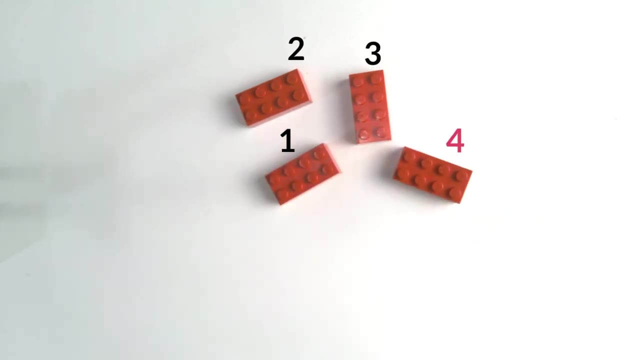 Okay, But if I do move them around, like I could even move them kind of like this: Yeah, it's still four. Okay, Can you count to make sure: One, two, three, four, Four Legos, That's right, Very good, All right, Now we're going to do a quiz. 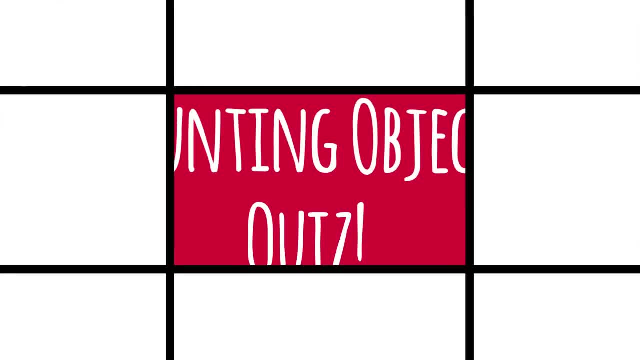 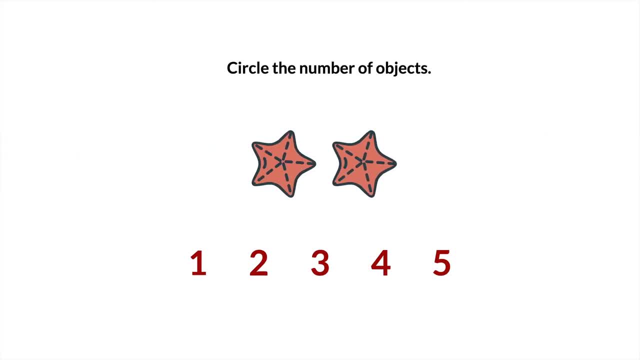 I love quizzes. Are you ready to do it? Yes, Okay, So I'm going to show you some objects on the screen and then you're going to count them. All right, Look at that Sea stars. You like sea stars, right? 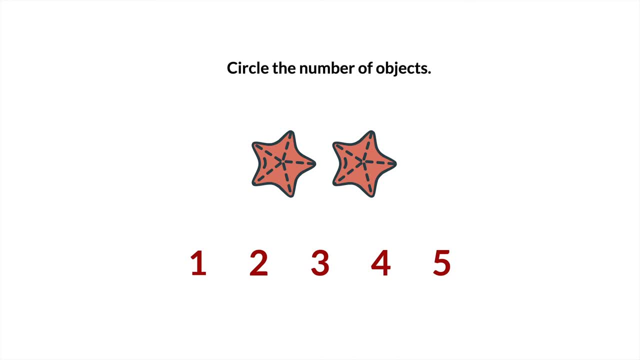 Yeah, because I studied them. Okay, All right, So you're going to count those and you can touch them using the screen, and then you're going to circle the right number: Easy: One, two, Two. what Sea stars? And you circle the number two. 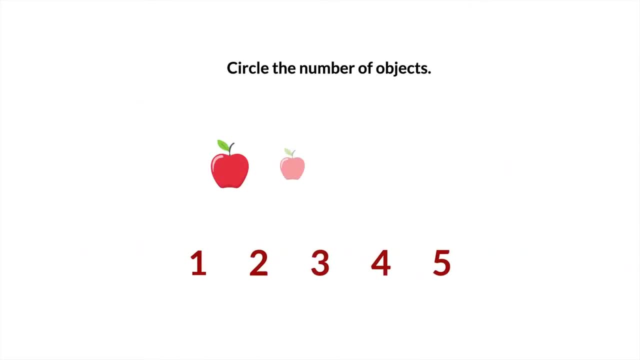 All right, Next set of objects. What are those Apples? Four to be exact. One, two, three, four, Four apples, Good job, Okay, Next set of objects, And I think you're going to like this one. 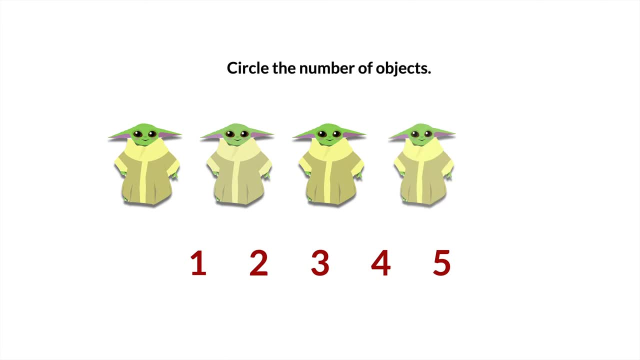 Baby yodas. So cute, They are cute, But how many are there exactly? Five, One, two, three, four, five, Five baby yodas. Good job, Okay. So I've got a question for you. 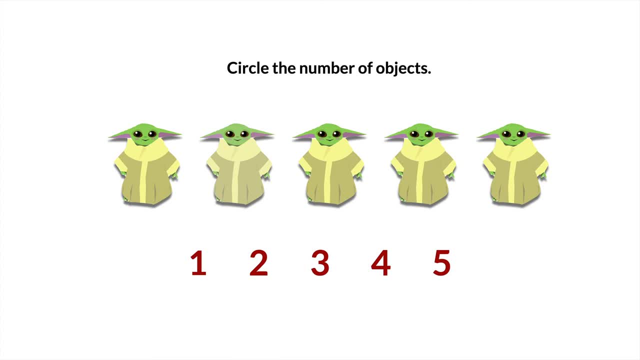 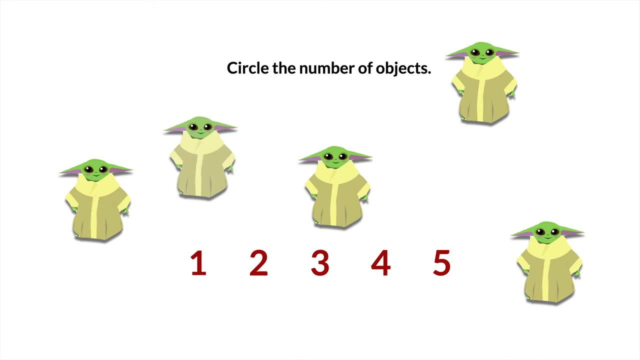 What is it? What happens if the baby yodas move around? Well, it's still five. One, two, three, four, five, Five baby yodas. Excellent, Okay, Really good job counting today. Dylan, You know, I think you're a lot better now than I was when I was your age. 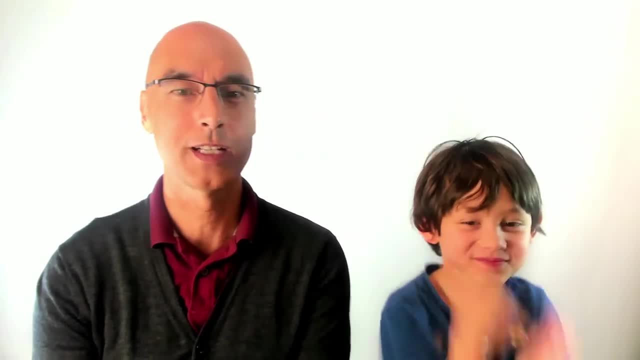 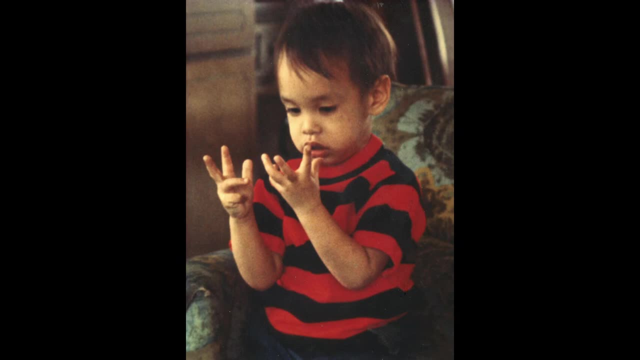 You want to see a picture of me when I was counting? Of course I did. Okay, There it is. You look very confused. I think I was a little confused. Do you know actually, like how you used to count when you were really little? 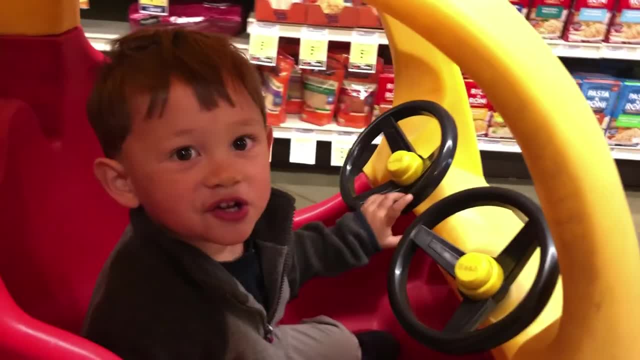 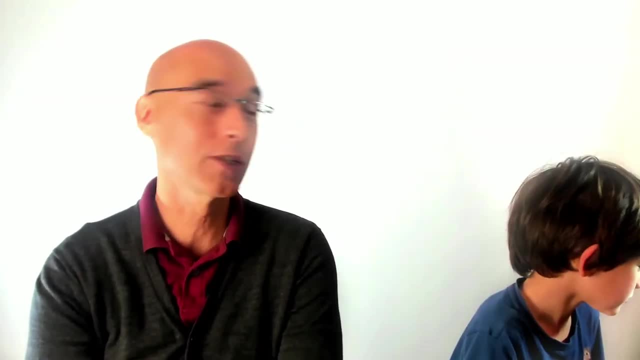 No, You used to go: Oh yeah, Two, nine, two, nine, two. Yeah, Those were the only numbers you knew: Two, nine, two, nine, two, nine. You couldn't get to 10.. But that's okay. Now you're really good at counting. 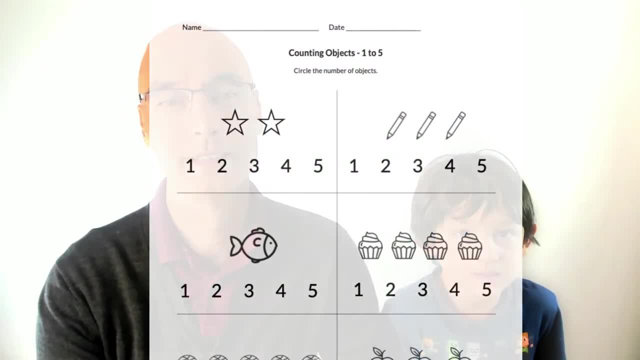 One, two, three, four, five, six, seven, eight, nine, 10,, 11,, 12,, 13,, 14,, 15,, 16,, 17,, 18, 19.. Okay, So if you want to practice some of the counting, then you can find a worksheet. that's down below in the description of this video. 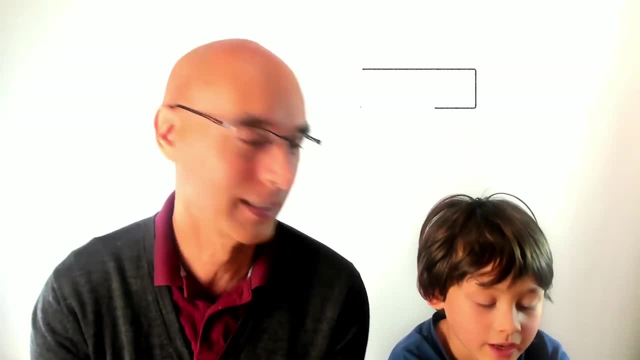 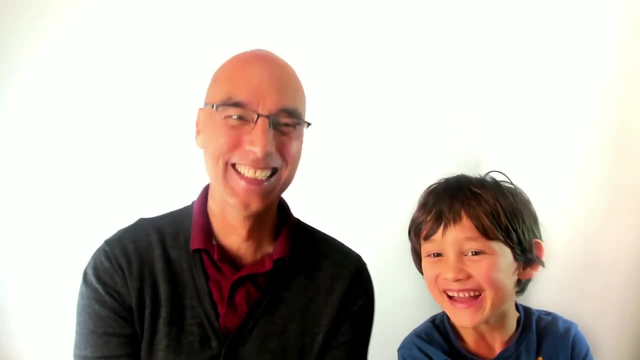 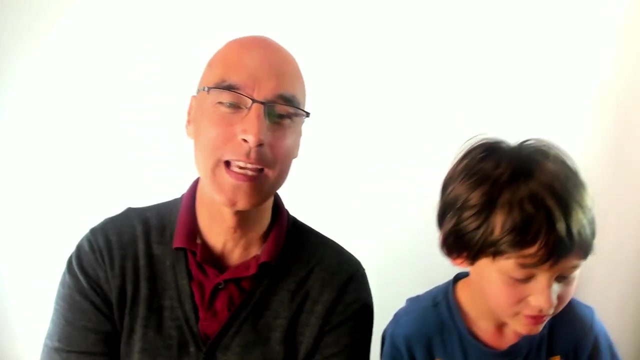 If you liked this video, make sure that you Hit the subscribe button and tickle the notification bell. Tickle the notification bell. Yeah, I just said that because sometimes when they say that, they actually say tickle the notification bell. Okay, All right, So tickle the notification bell.